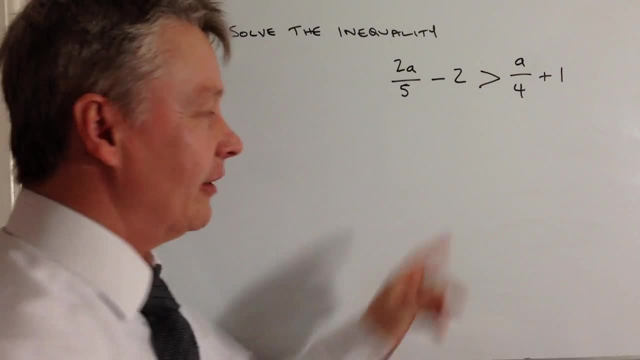 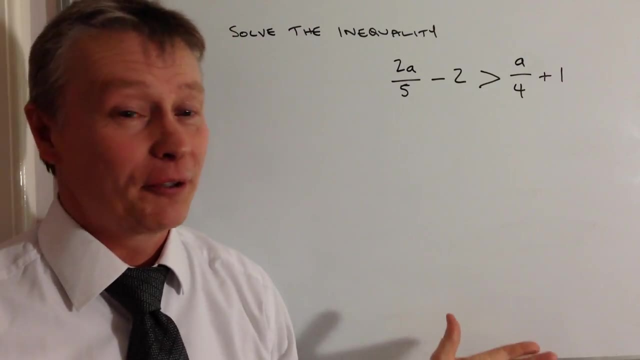 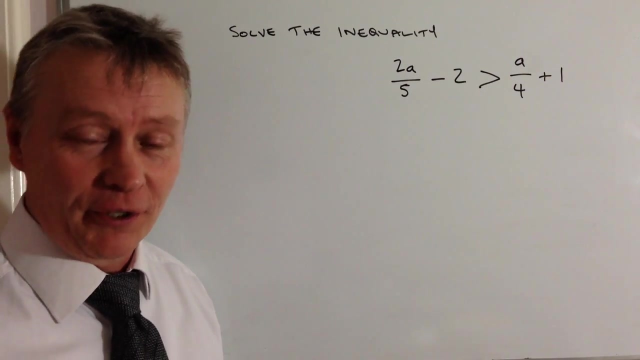 So, effectively, you've got a fraction here and a fraction here, and this is an equal sign in the middle. So whatever we do to the left hand side, provided we do it to the right, then we're okay. So in this case I've got a 5 and a 4, I'm going to multiply through by the lowest common multiple. 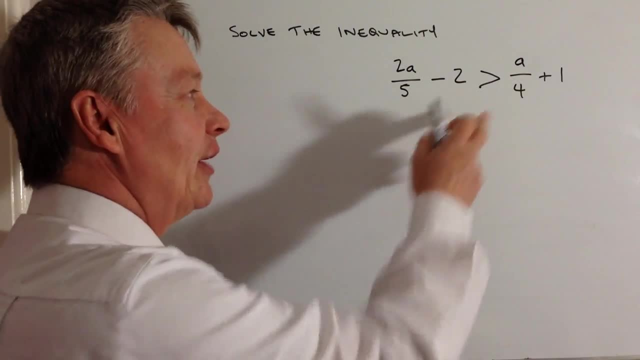 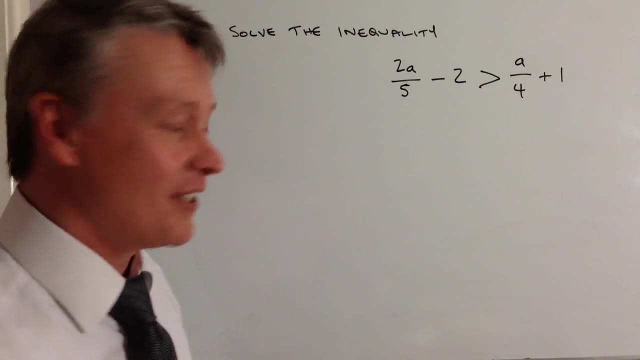 And that'll just make my life a little bit easier, because then I can get rid of the 5 and the 4.. What I mean by that is: the lowest common multiple of 5 and 4 is 20.. So I'm going to multiply both sides by 20.. 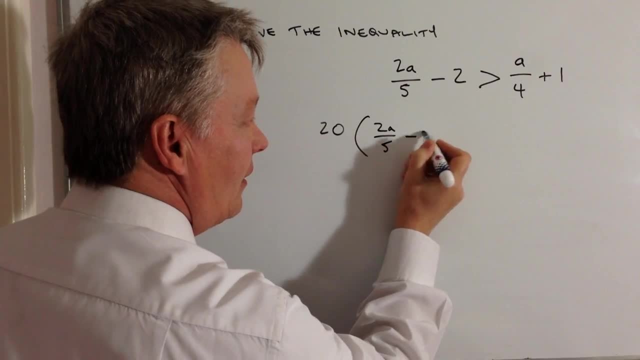 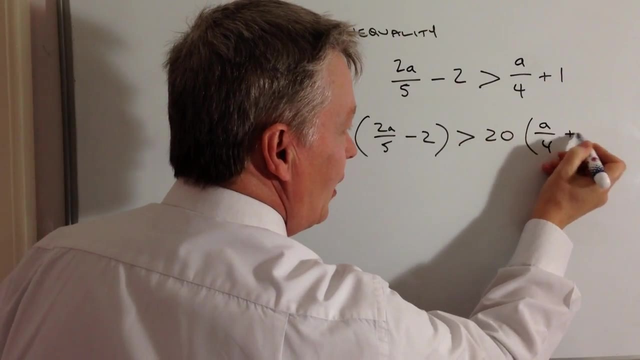 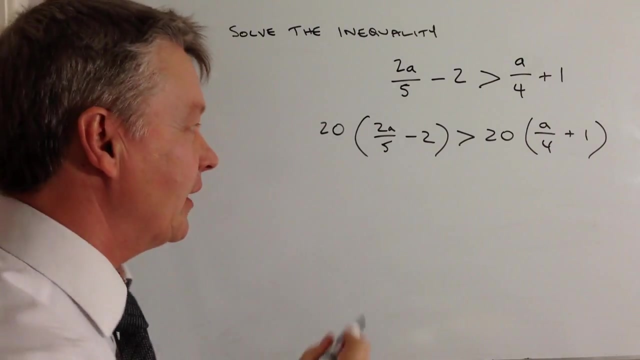 And I end up writing this: okay, and I'm going to multiply that side by 20 and that's going to be a over 4 plus 1.. And then it's really just a case of multiplying out the brackets. Now, if I multiply out the brackets for this one here, I'm going to multiply that 20 times 2a over 5.. 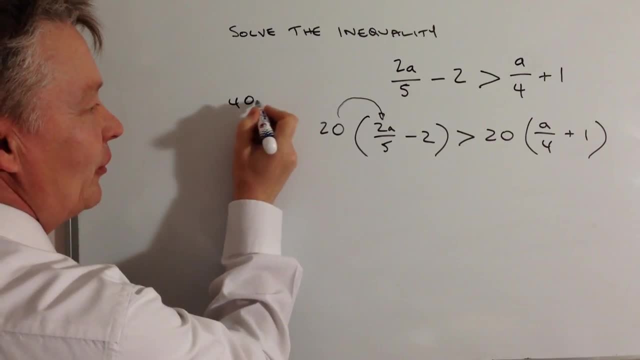 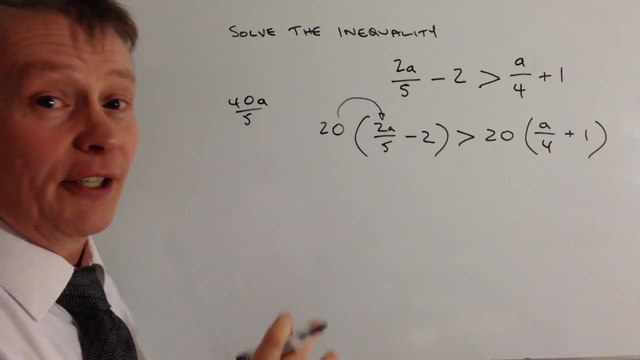 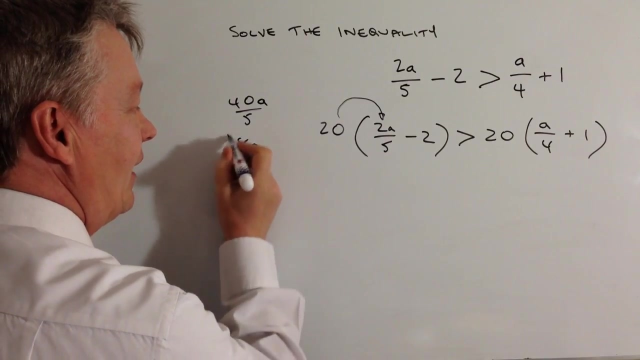 And what I really get with this is 40a. so 20 times 2 is 40a divided by 5.. And what I can do is I can simplify that down to 5 into 40 is 8,, so that becomes 8a. 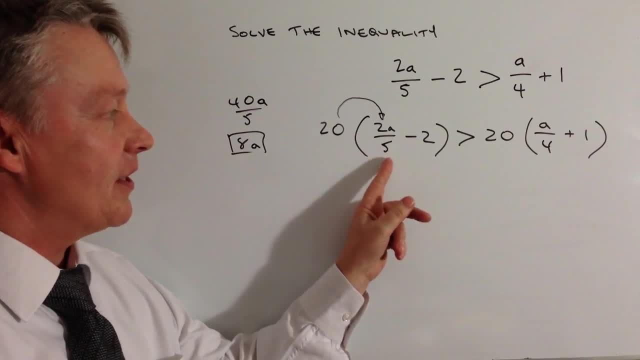 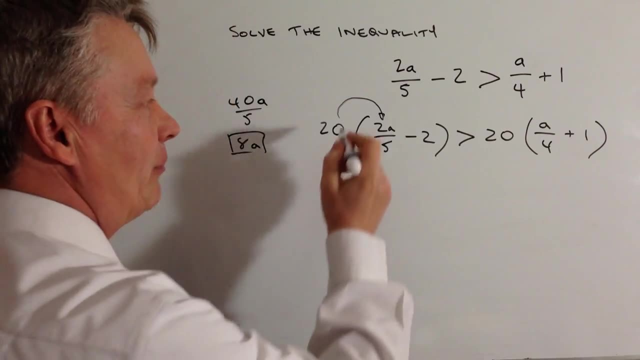 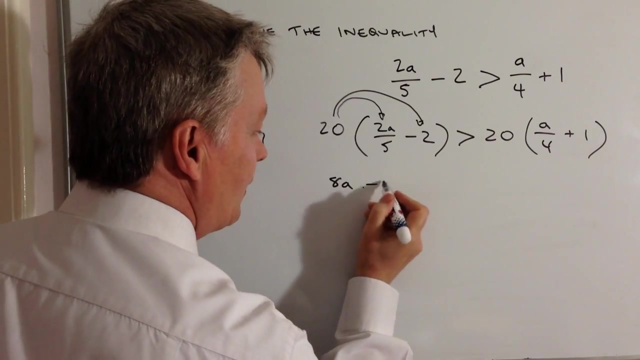 And that's brilliant, because it means, then, that I lose this denominator over here. So this first term will become 8a, And then my second term will be 8a, And that will become 20 times minus 2.. Well, that's going to be minus 40.. 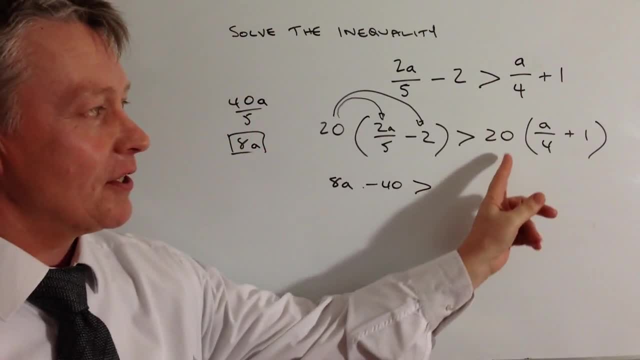 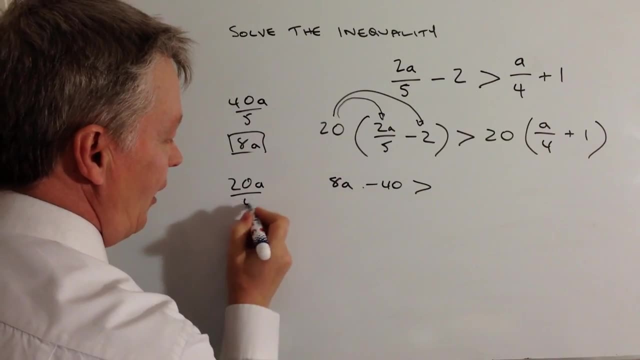 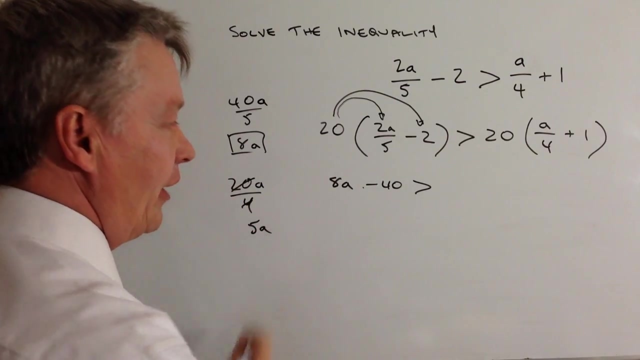 And that's going to be greater than. And then I've got a similar situation here where I've got 20 times a over 4 becomes 28 over 4.. Well, I'm going to simplify that a little bit further: divide through by 4, and that becomes 5a. 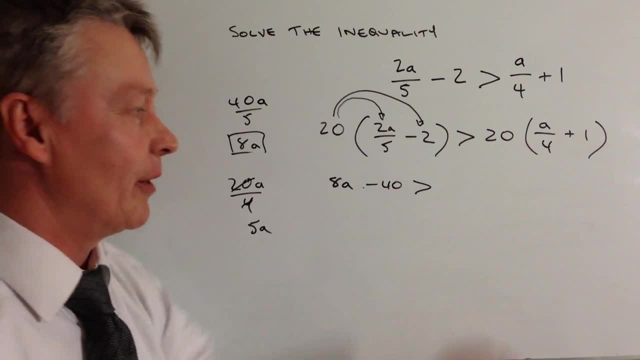 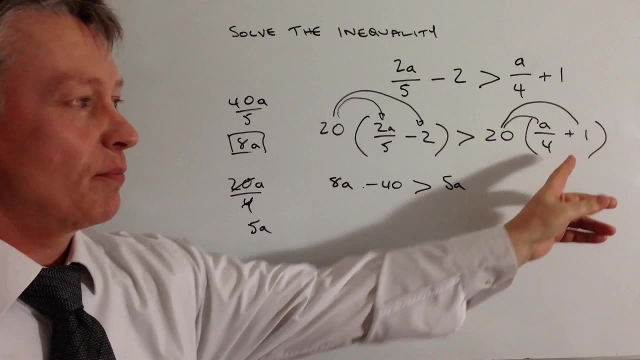 Well, that's excellent again, because again I've lost the denominator, So that becomes 5a. So that's that one there, And then this last one will be 20 times plus 1, but that's going to be plus 20..